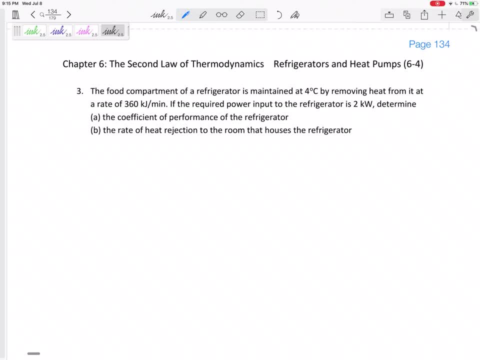 Alright, so this will work out some problems with coefficients of performance, work, heat transfer for refrigerators and heat pumps. A lot of this is just units and unit conversions And also figuring out what the problem statement is really telling us. It tells us 360 kJ per minute. What is that? It tells us 2 kW. What is that? 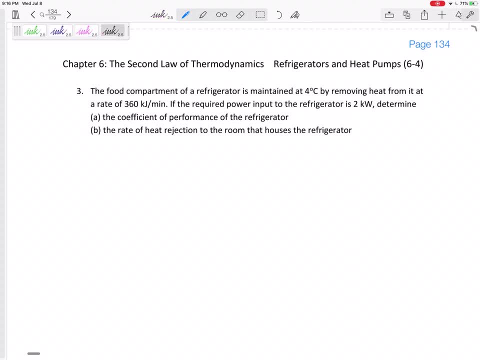 Alright, so let's read this. Food compartment in a refrigerator is maintained at 4 degrees Celsius by removing heat from it at a rate of 360 kJ per minute. What is that? That is the rate of heat that we are removing from the colder stuff on the inside of the refrigerator. That is QL And it's a rate. It's not just kJ per minute. So that's a QL dot. 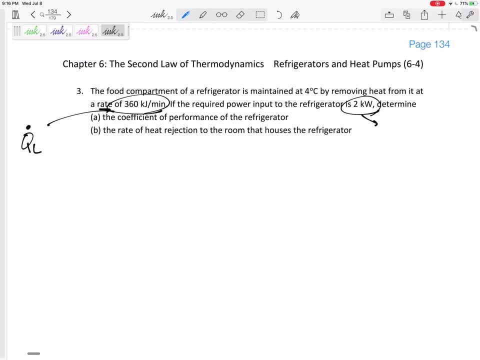 Alright, if the required input to the refrigerator is 2 kW, that's WN or WnetN. Determine the coefficient of performance of the refrigerator and the rate of heat rejection to the room. So we want to find COP, subscript R, And we want to find what is this? The rate of heat rejection to the room, That's QH dot. 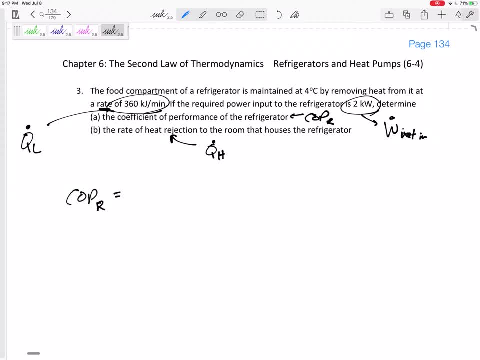 Alright. so we have a few equations. We have equations for coefficient of performance for a refrigerator. One of them is QL dot over WN dot. So this is just 360 kJ per minute over the work in of 2 kW. Now this coefficient of performance is unitless. These units don't exactly work out. What is a kW? A kW is a kJ per second, So I need to convert minutes to seconds. Let's see. So yeah, dividing it by 60 would be 60 kW. 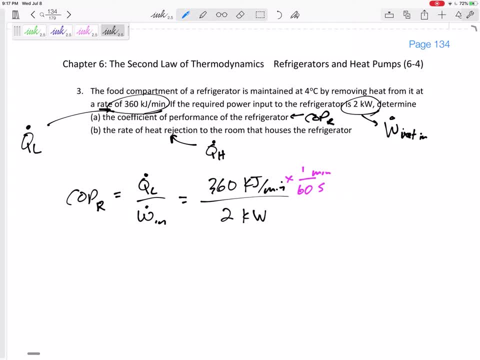 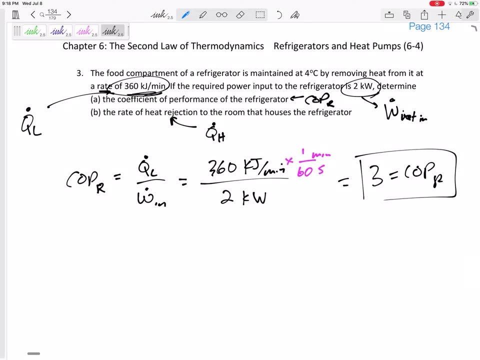 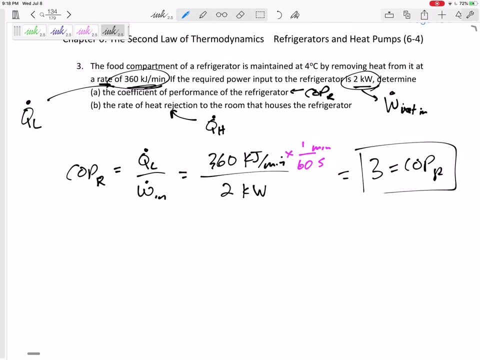 So 6 over 3.. So yeah, this would be 3- is the coefficient of performance of this heat, of this refrigerator that is removing QL at a rate of 360 kJ per minute And it's taking a power in of 2 kW, And then part B, the rate of heat rejection, QH. So let's see. I've got a couple of equations. 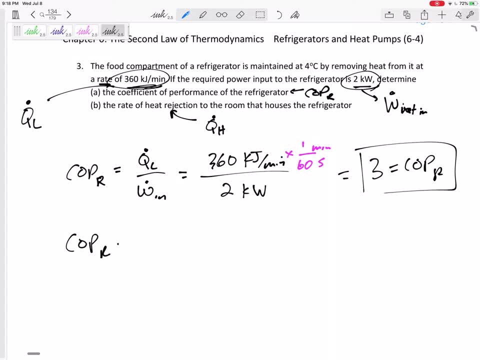 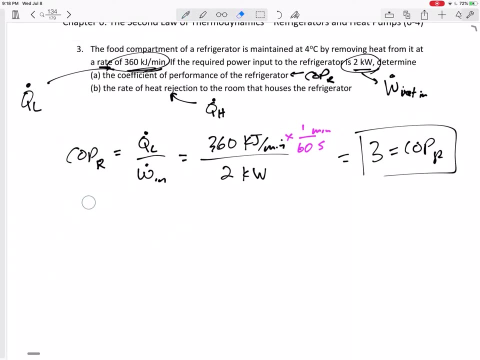 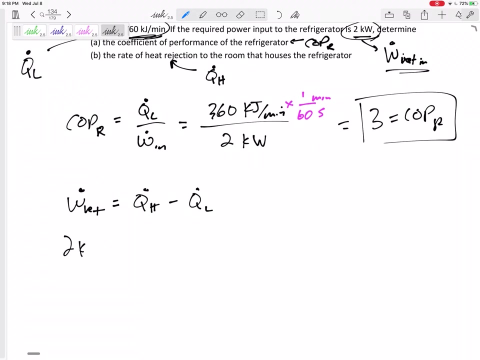 I could, I could. now that I've found COP, I could say COP is QL over QH minus QL, So that's one. And since I know those, I could find QH. Or that would actually be going around the block, doing too much work. I know the work, the net work, And I know that the net work is QH minus QL. Or in this case, these are dots right, These are times, rate of change or power. So 2 kW. 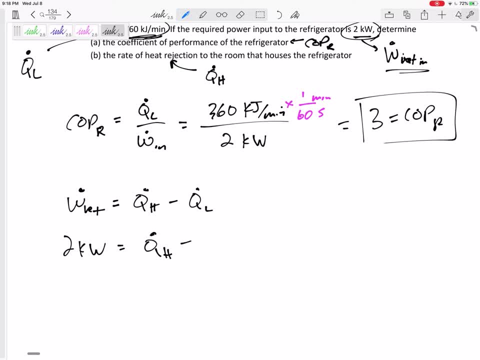 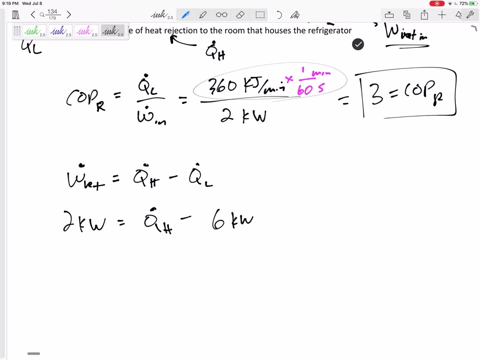 Is equal to QH that I'm looking for, minus 360 divided by 60, right, Minus 6,, uh, minus 6 kW, right 360 divided by 60. So here, QH is 8 kW. QH is the rate of heat rejection to the room that houses the refrigerator. 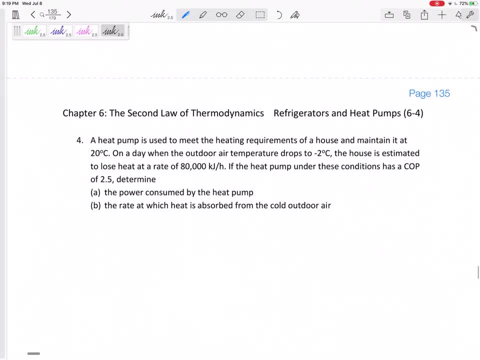 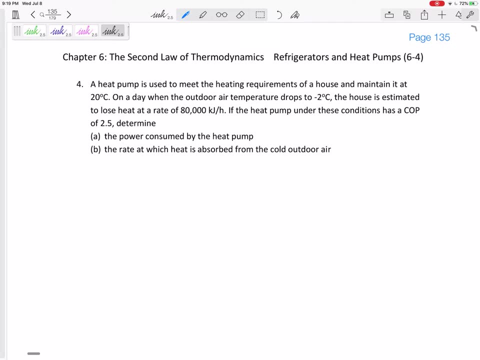 Okay, Not too bad. Just a little bit of units right there. Let's do another one real quick, All right. Heat pump is used to meet the heating requirements of the house, Maintain it at some a certain temperature. On a day when the outside temperature drops to negative 2,, the house is estimated to lose heat at a rate of 80,000 kJ per hour. 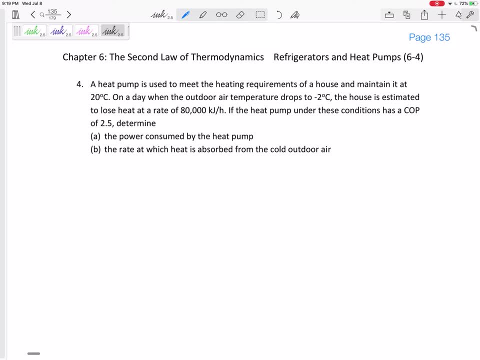 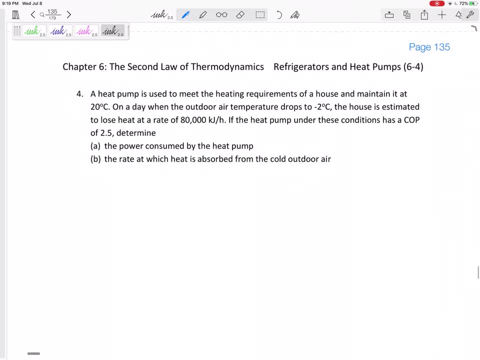 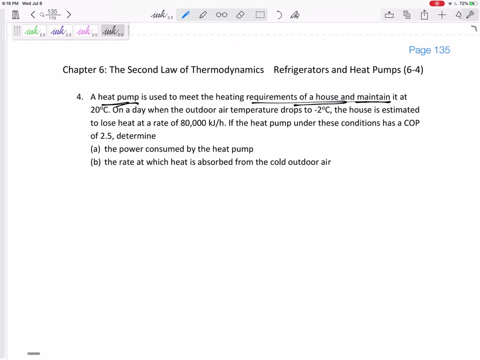 If the heat pump, under these conditions, have a coefficient of performance of 2.5, determine the power consumed by the heat pump and the rate at which heat is absorbed from the cold outside air. Okay, So A heat pump maintains a house at a certain temperature. 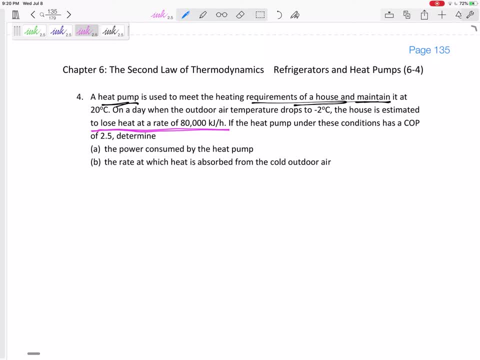 So let's see, They kind of told it to told this to us in a roundabout way. If the house is losing heat at a rate of 80,000 kJ per hour, but I want to maintain it at a constant temperature, what should the heat pump do? 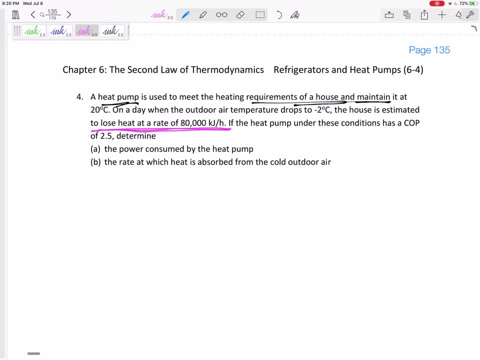 The heat pump should be pumping heat back into it At the same rate. it is losing It this. right, there is their way of telling us the QH of the heat pump. right? The house estimated that it's losing 80,000, but if you want to keep it at a constant temperature, we've got to be replacing that 80,000.. 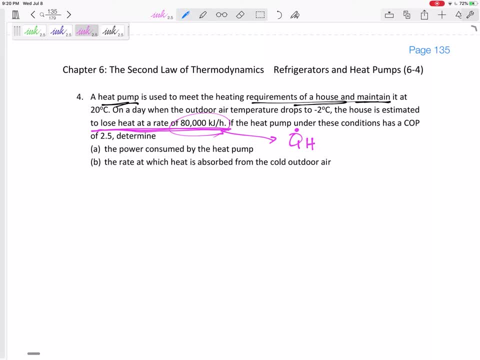 The heat pump does that. The heat pump pumps in 80,000 kJ per hour to keep it at a certain temperature. So if we know QH, if we know COP, can we find everything else right? Can we find everything else? 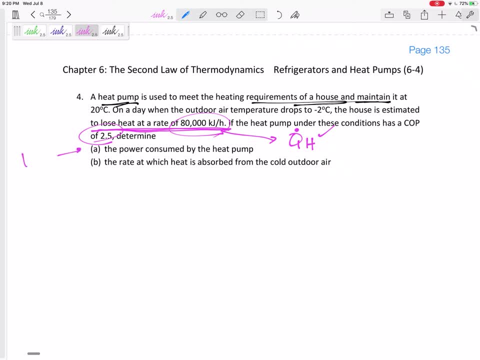 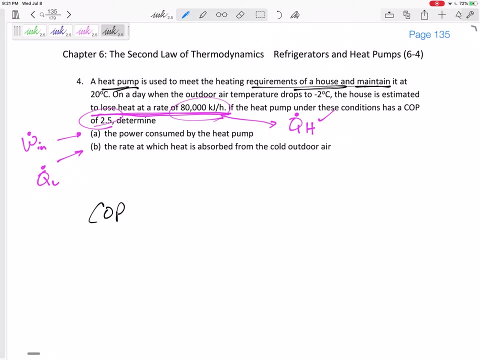 Can we find: A- the power consumed, the W net in B- the rate at which heat is absorbed from the cold outside air? that is QL dot. That is QL dot. All right, So there might be better ways, might be more efficient way, or maybe efficient is a better term. 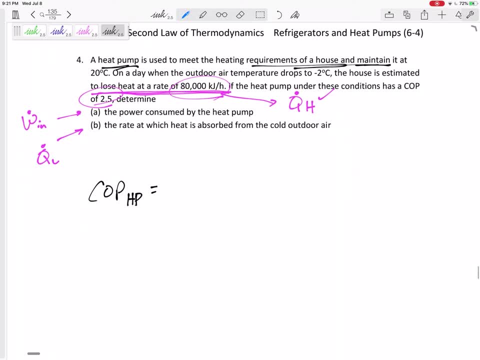 There are a lot of different equations and sometimes you can use different equations, go about these differently, take a different route than me, All right, but I know the coefficient of performance is 1 over 1, minus QL over QH. 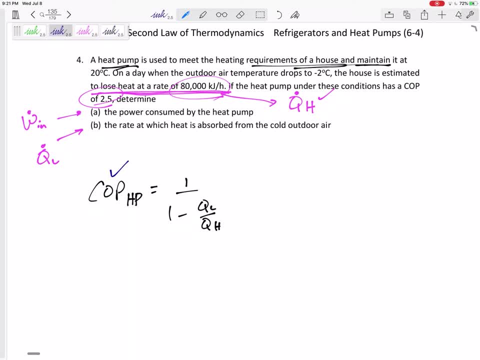 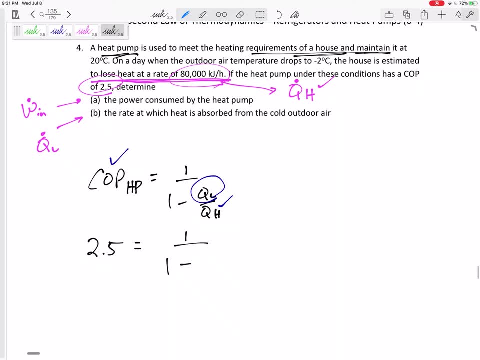 So if I know coefficient of performance and I know the QH, I can find the QL right. This is 2.5, 1 over 1, minus QL over 80,000 kJ per hour. Maybe I could change that to kilowatts, but if I don't change anything, 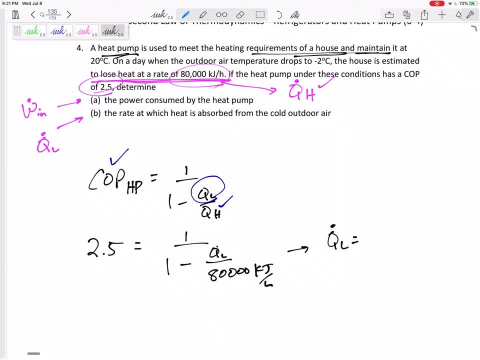 then I'm going to lose 80,000 kJ per hour, So I'm going to be left with a QL of 48,000 kJ per hour. It didn't tell me what units it wanted, So I actually saw B first. 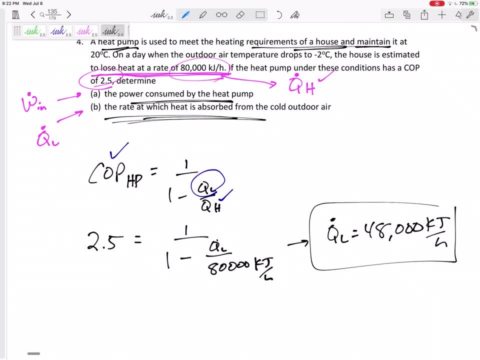 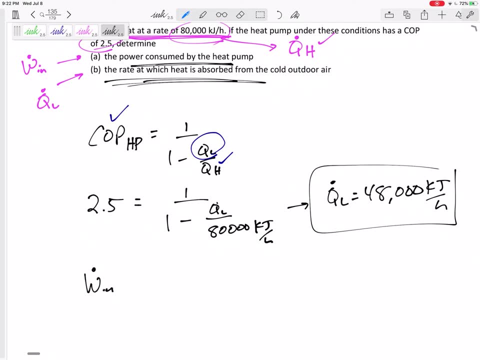 It didn't tell me that it wanted it in kilowatts, So I guess I'll just leave it as kJ per hour, And then I need to find the power, the W net in. Well, that's QH minus QL. 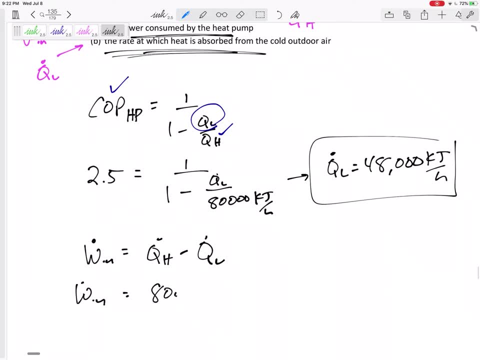 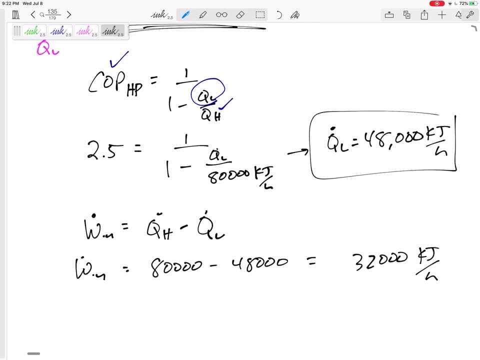 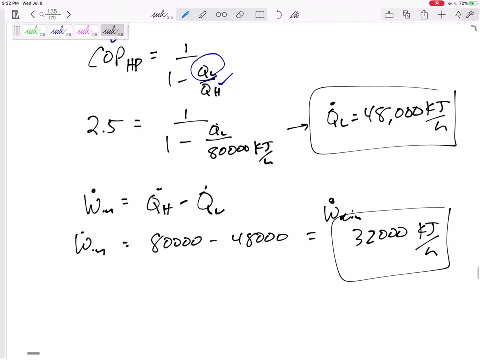 I have both of those now. W net in 80,000 minus 48,000, 32,000 kJ per hour. That would be the W net in the power in. Okay Yeah, All right, So there we go. 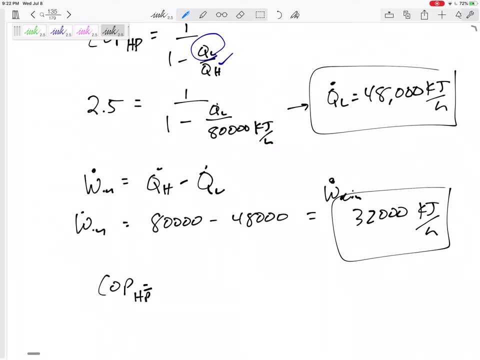 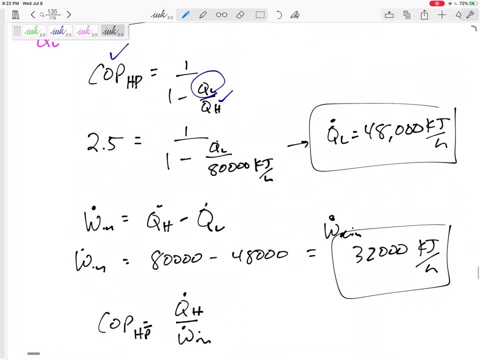 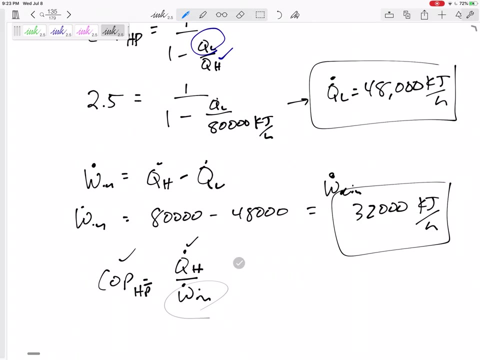 I probably could have done. COP is QH over 20. Or W in. I might should have started with that one. If I know COP, I know QH. Yeah, That's probably the way I should have done that. But you can see we can take different routes to get there. 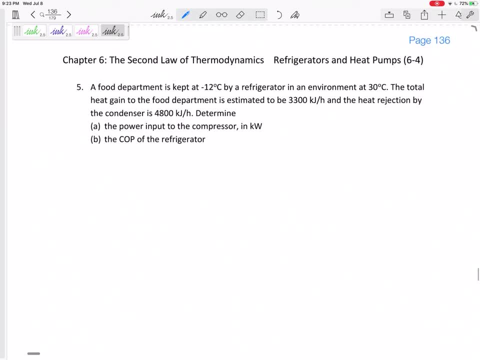 Let's do one more quick one. One more quick one. All right, Food department is kept at negative 12 degrees Celsius by our refrigerator in an environment of 30 degrees C, So this is kind of a freezer right, But still the same idea. 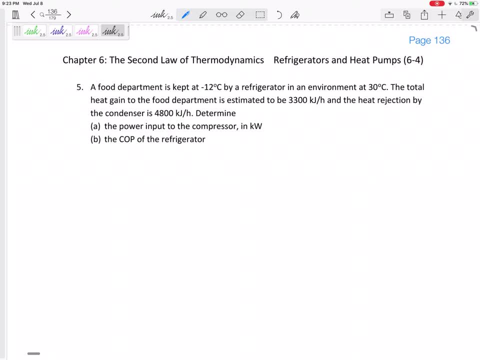 So the total heat gain to the food department is estimated to be 3,300 kJ per hour And the heat rejection by the condenser is 4,800 kJ per hour. Do you see that? That is the heat rejection to the outside air. 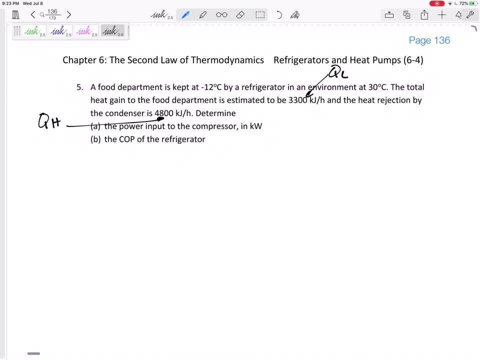 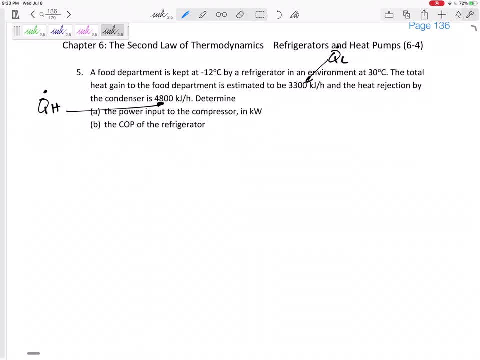 That's the QH. This right here is the QL. Yeah, not too bad. So let's determine the WN in kilowatts and the coefficient of performance of the refrigerator. All right, So the WN is QH minus QL. 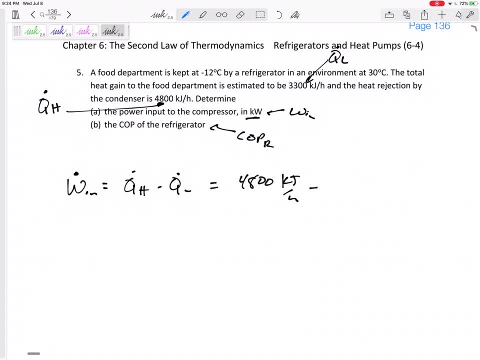 So 4,800 kJ per hour minus 3,300 kJ per hour. I'll go ahead and say I get 1,500, but that's not kilowatts, That's kJ per hour. I need to change hours to seconds. 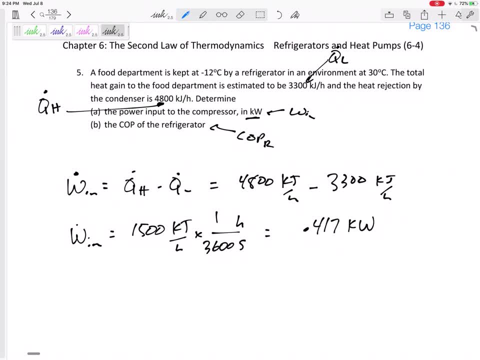 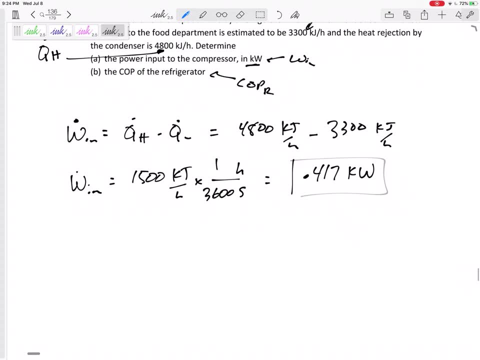 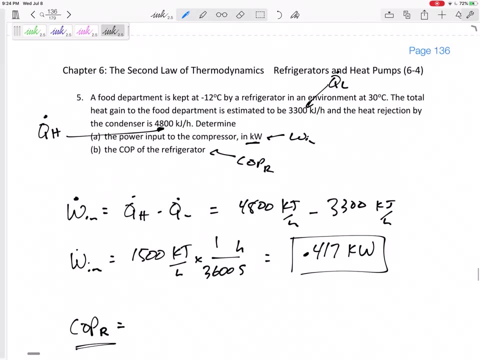 Divided by 3,600.. So 0.417 kilowatts is the work in the power input in And part B, the coefficient of performance. A number of equations I could do And be careful. Coefficient of performance for a refrigerator is different than the coefficient of performance of a heat pump. 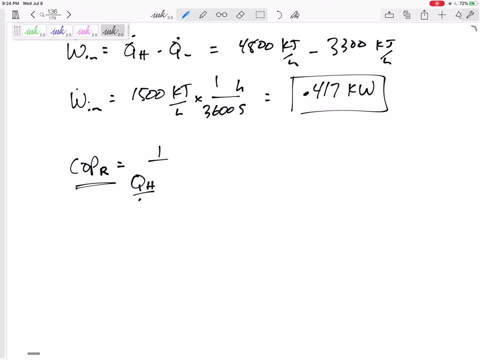 Coefficient of performance of a refrigerator: 1 over QH over QL, So 1 over QH over QL, So 1 over QH over QL Or QL over WN. Yeah, that would be easier. 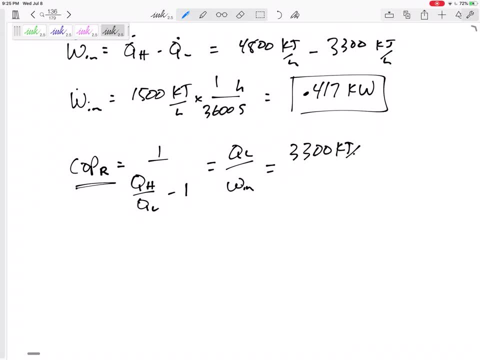 I've got this as 3,300 kJ per hour. over 1,500 kJ per hour Units cancel out. This is 2.2.. Coefficient of performance of my refrigerator is 2.2 right here, So you see that there's.